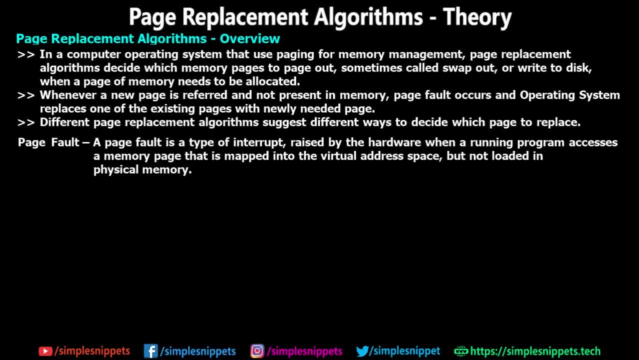 fault happens and how to handle page faults. So if you have missed those videos, you can check those videos in this playlist. And if you already know what is paging, what is page faults, the next thing that comes is page replacement algorithms. So this is going to 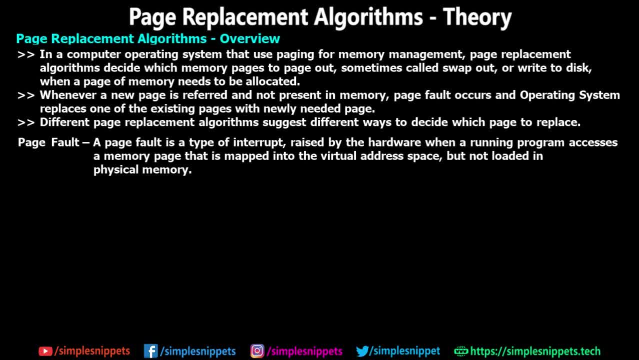 be a very quick, short video because it's going to be theory and we are not actually solving any numericals based on a particular page replacement algorithm. that will be in the next video, But this video is all about the theory of why we need page replacement and when do we. 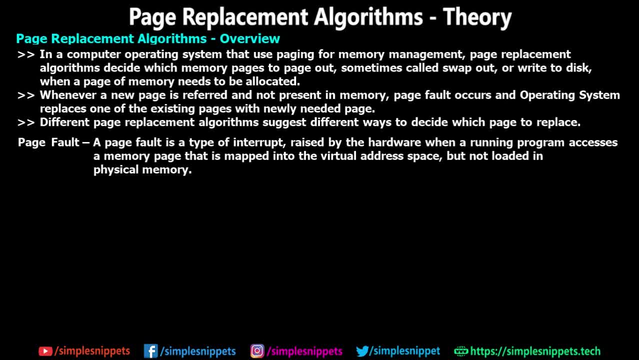 need page replacement. So if you already know about this, you can skip to the next video, wherein we discuss the individual page replacement algorithms and solve numericals. So, with that being said, let's start off with today's topic. So, as you can see on the screen, I have a 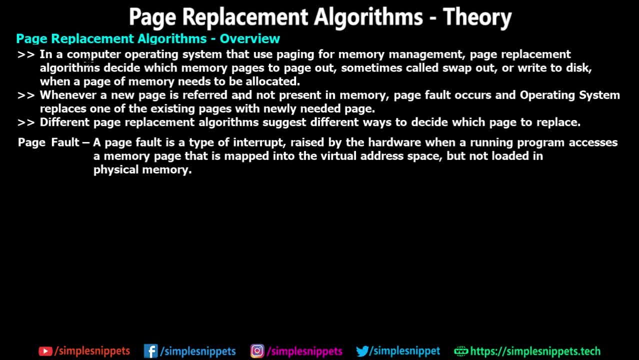 little bit of theory about what page replacement algorithms are So in computer operating systems that use paging. so whenever a paging memory management scheme is implemented in any kind of operating system or in any kind of software, you can use paging to solve numerical problems. 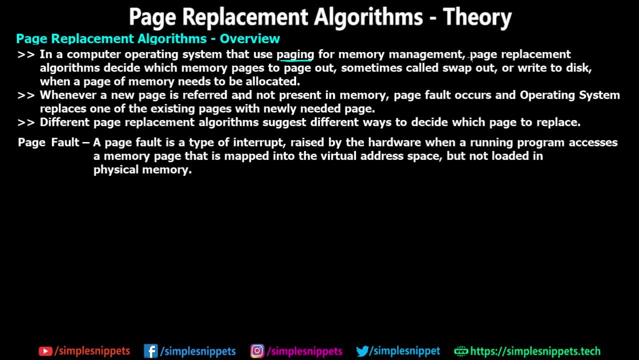 So let's start off with paging. So paging is a kind of computer system for memory management. The page replacement algorithm decides which memory pages to page out- sometimes called swap out, or write to disk, and when a page of memory needs to be allocated. So what this? 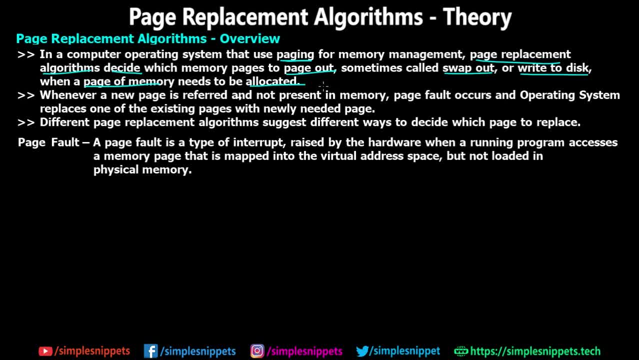 means is these algorithms basically dictate how and when a page is supposed to be removed from the physical memory and shifted to the virtual memory, and vice versa. Okay, So when a new page is referred and not present in memory, and this memory is the physical memory, 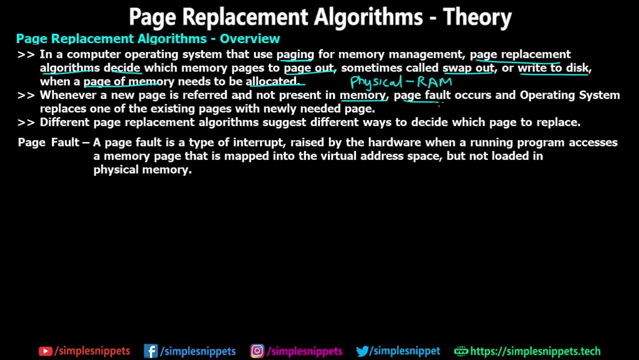 or you can also relate it with RAM. So page fault occurs and operating system replaces one of the existing pages with newly needed pages, or it adds the page in an empty frame. Okay, So there are two scenarios. Either your memory is full and you have to replace a page. 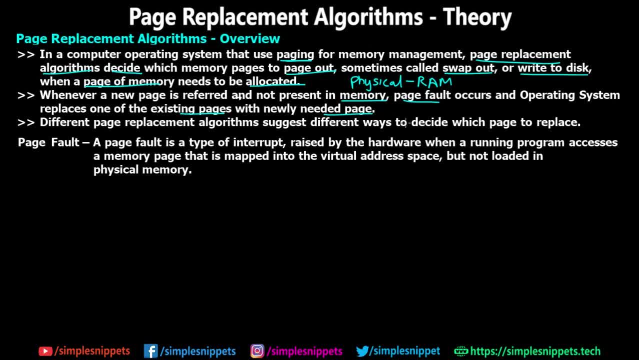 with another page or your memory is not full, So you have to find an empty frame and add that page from the virtual memory into that frame. Okay, So different page replacement algorithms suggest different ways to decide which page to replace. So that's where the 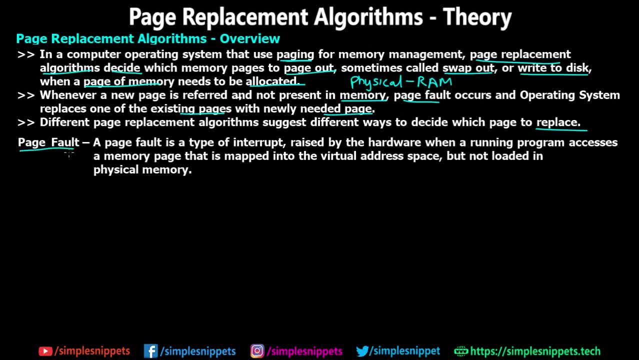 different page replacement algorithms comes into picture And you already know what a page fault is right. So this is a big definition and it's a very, what we say, jargon filled definition. but in simple words, page fault happens when the page is not found in the 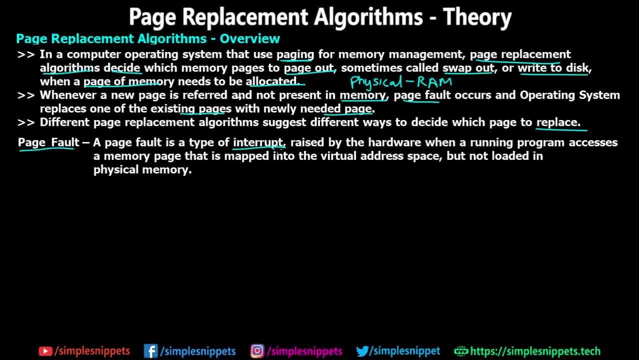 physical memory and then a page fault interrupt is generated. So interrupt is a signal which we saw in the previous video, which is a high priority signal to the OS, which states that it requires that necessary page from the virtual memory into the physical memory. Okay So, 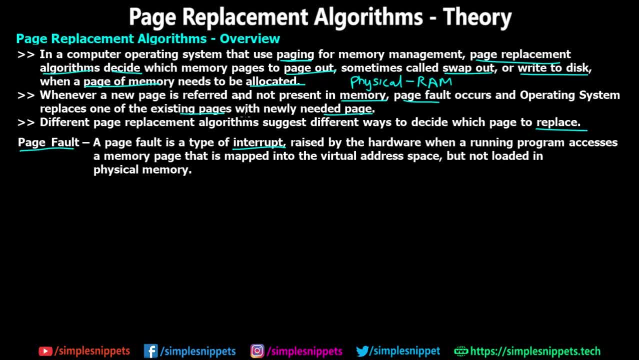 this was a little bit of theory. If you are making a page replacement algorithm and you want to replace a page with another page, you can use a page replacement algorithm. You can also use a page replacement algorithm to replace the page. So let's take a scenario. So consider a process, a, divided into five. 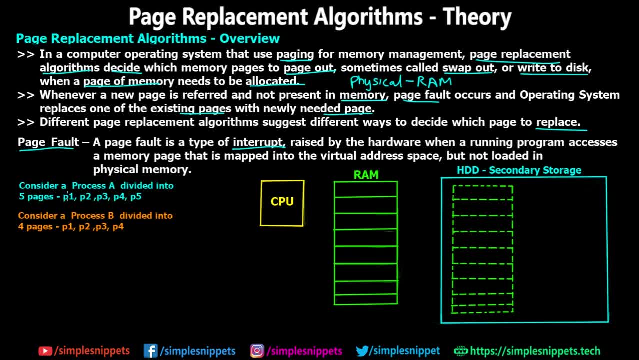 pages P one, P two, P three and P four. Okay, So let's say process a is started or initialized first, So it's loaded in the Ram. So you can see our physical memory Ram over here. So I'm just going to allocate P one, P two, P three, P five and P four. Okay, So now. 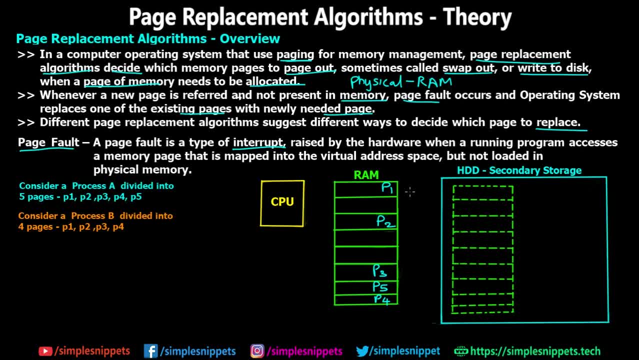 the order doesn't matter. right, So we can have non-contiguous memory allocations using scheme. right, because where exactly the page is is maintained by a page table. right, so we have a page table in between which maintains the page number and frame number. so i'm not going to get into a 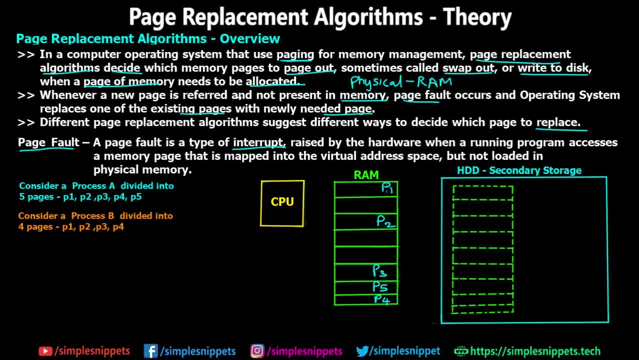 lot of detail. as of now we're just taking an overview. so all the pages of process a are loaded in the ram. so let's say cpu is executing p1, that is page 1 of process a right now. now consider a process b which comes into the ram. so a process b is initiated and it has four pages, right. so 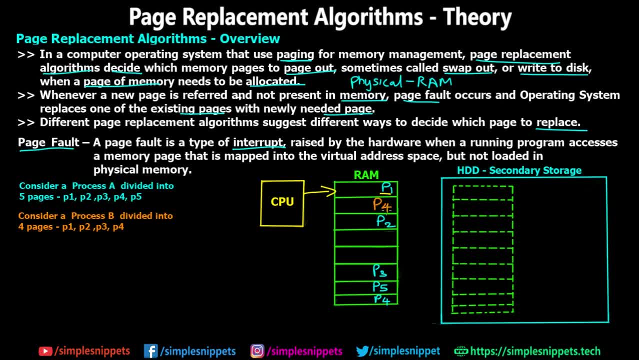 let's load these pages in the memory. so i'm gonna say p4, p2, p3, but now you can see p1 cannot be loaded in the ram because our ram is full. so let's assume our ram is very limited and it's full now. 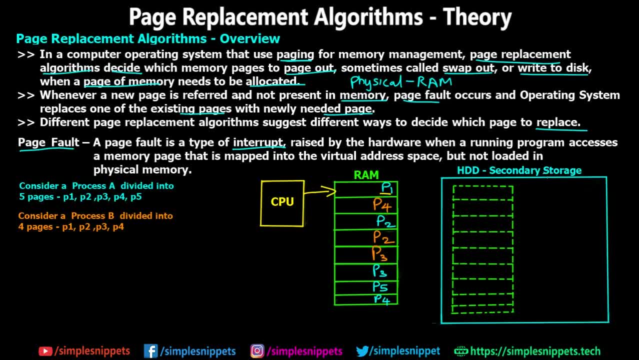 so in paging we know that some portion of the secondary storage can be used as virtual memory, vm. i'm just writing short forms. this is virtual memory. so let's say p1 is stored somewhere over here in virtual memory. now cpu moves on to process b. okay, and 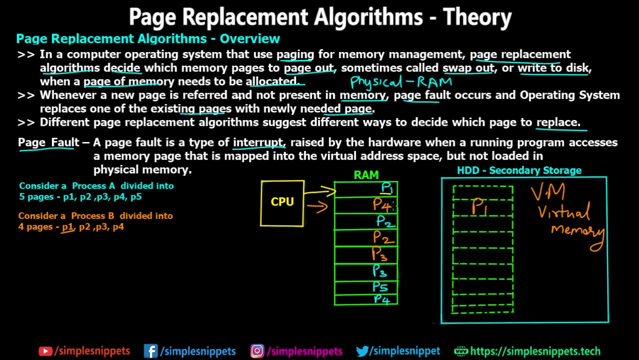 first page. p1 is not there in the ram right. so the mmu looks up in the page table of process b and sees that for p1 there is an invalid entry. so that is a page fault right. since there is no entry for p1 in the process table of process b, an interrupt is generated and the operating system